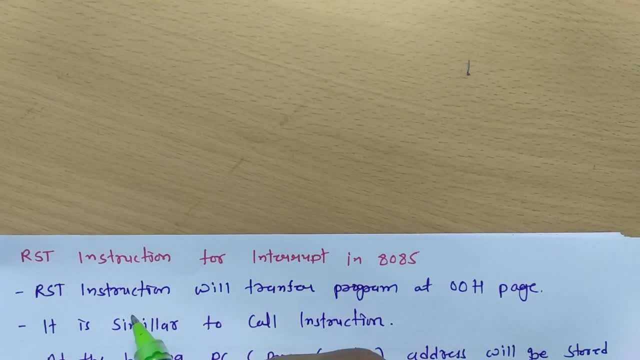 What is RST instruction And then I'll explain complete process with one example, so it will be more clear. Now see RST instruction. that is what we are utilizing: it to transfer control to 00Hacks page And that is what I have already explained in previous session. To provide service. to interrupt RST instruction will be executed and that will transfer program control to 00Hacks page. It is similar to call instruction At the beginning. 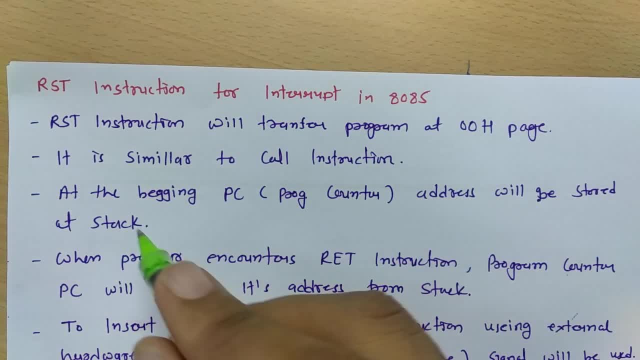 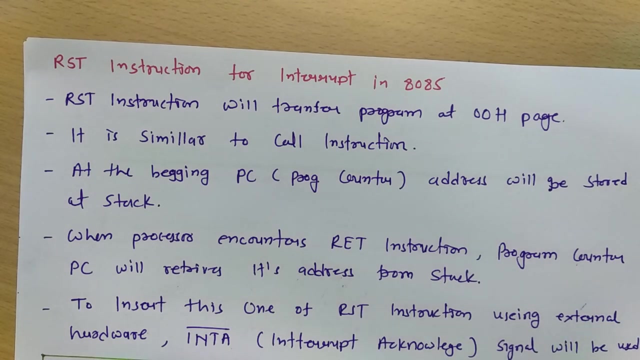 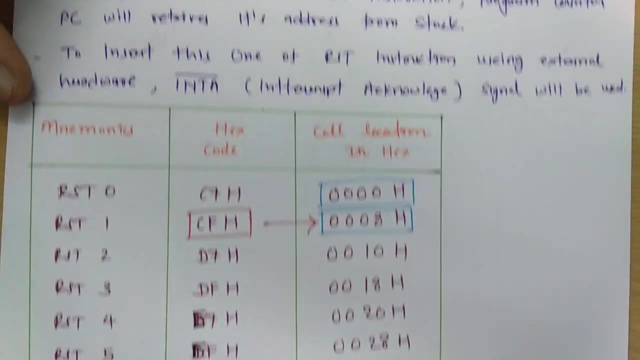 program counter address will get stored at stack And when processor encounters return instruction program counter again, retrieve original data from stack And to insert one of RST instruction external hardware that is using INTA bar signal. So let us see first what is RST instruction. So basically there are 8 RST instructions, RST 0 to RST 7.. 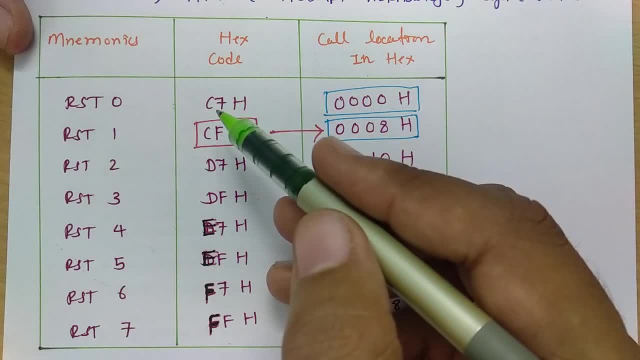 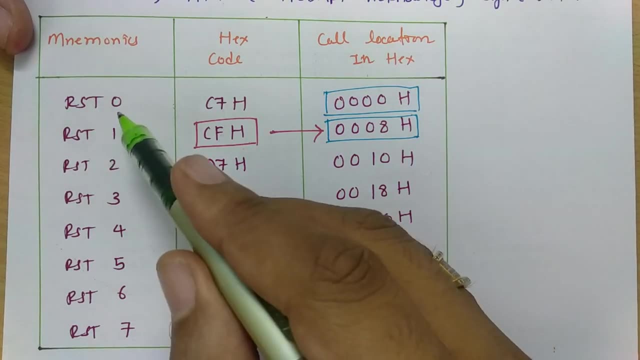 And HECCS code of these RST instruction, that is C7CF, He7DF, He7EF, F7, and FF. And when RST 0 instruction is getting executed, program counter will jump to location 0000 HECCS. 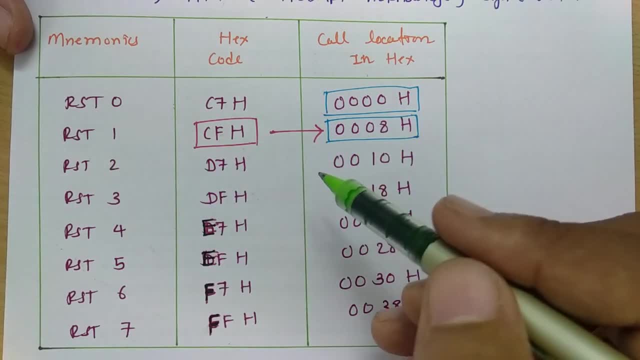 For RST 1, 0008. for RST 2: 0010. for RST 3: 0018,. for RST 4: 0020. HECCS. for RST 5: 0045. 00ате否. for RST 6: 0010. 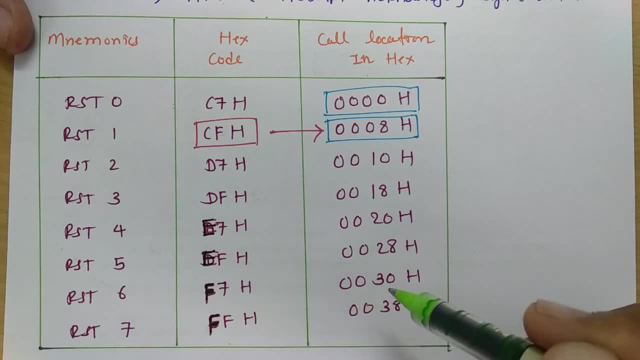 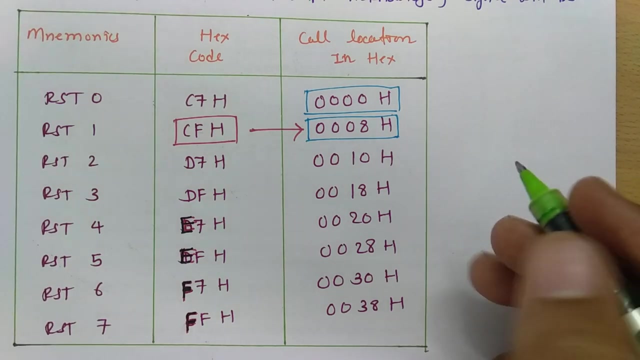 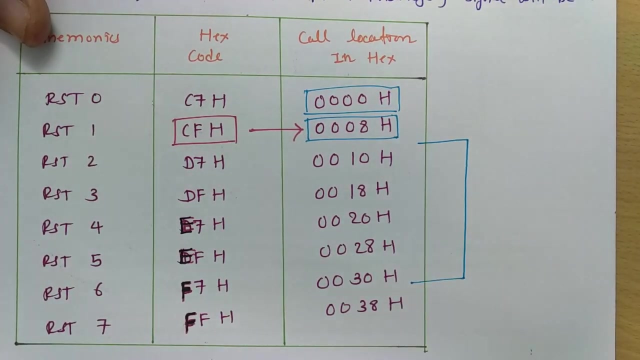 0028 hex. for RST 6: 0030 hex and for RST 7, program counter will jump to location 0038 hex. Now let us try to understand this: how this complete process will happen. So if I say here I have a processor, let us say this is processor and let us say this is device. 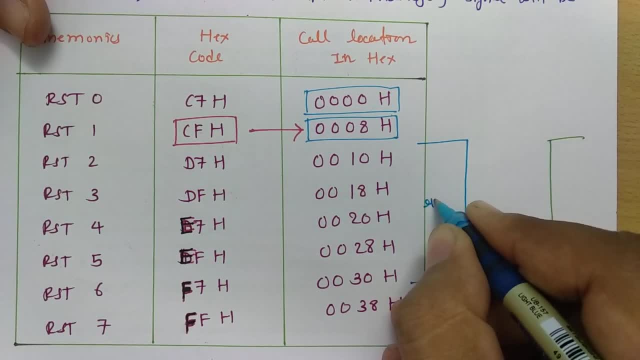 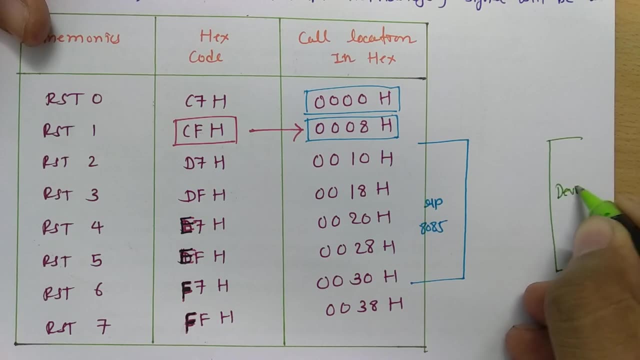 So here I have processor, here microprocessor 8085, and here I have a device. Now what happens is this device is sending interrupt request, So on INTR line, this device is sending interrupt request, So in acknowledgement of this request, microprocessor that will send interrupt acknowledgement to this device, So active. 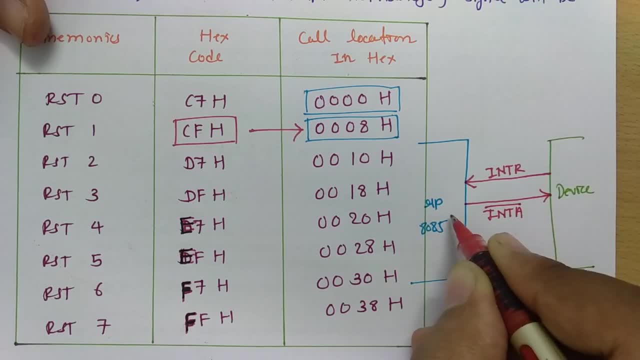 low signal. INTA bar: interrupt acknowledgement that will be given to this device. INTR that will be active high, so in counts I am writing 1 and INTA bar that is active low. So here, zero signal that will be given to this device. Now see, along with this INTA bar, what will happen is as this: 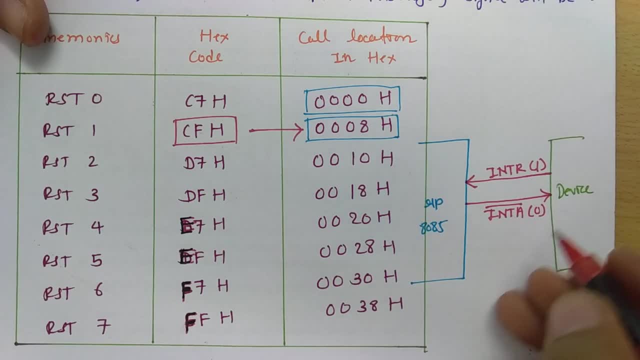 device is sending interrupt acknowledgement to this device. So here 0 signal that will be given to this device Now as it is sending HACKS to this device. If this device is receiving interrupt acknowledgement, this device, now it will forward HACKS code on D 0 to D 7.. So this device will send. 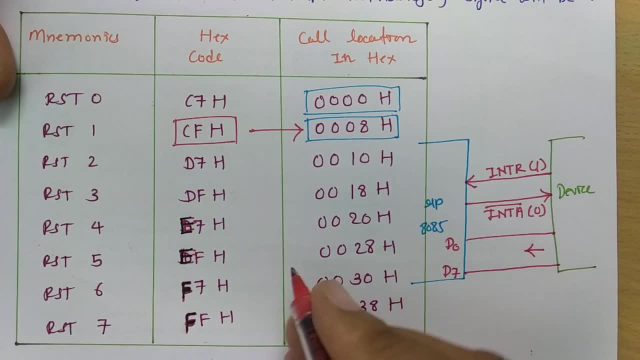 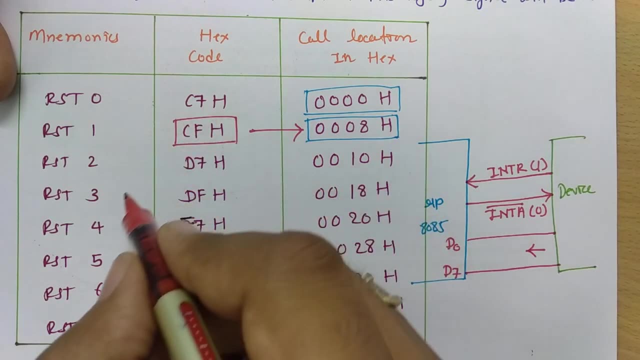 HACKS code on D 0 to D 7, and that HACKS code that could be any of this RST instruction. Now see, if I say CF, that is the data which I will be sending. So CF HACKS data if I send it on D 0 to D 7.. Now, if I say C, F, that is the data which I'll be sending. So CF HACKS data if I send it on D 0 to D 7.. Now you can see that all the 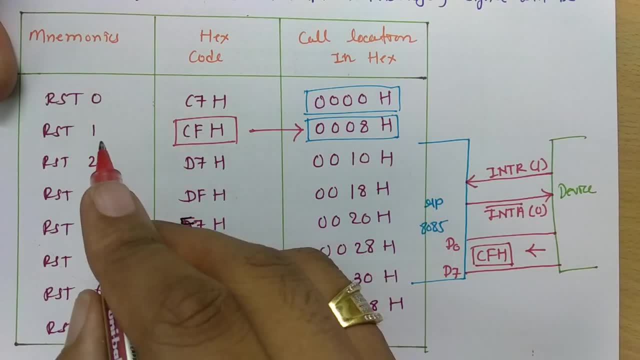 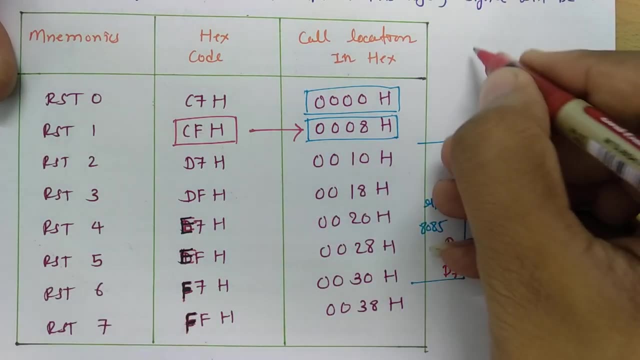 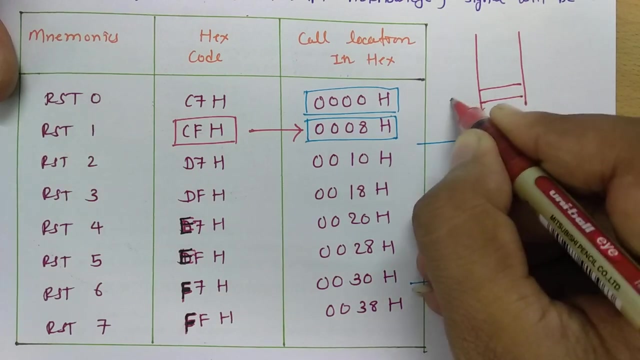 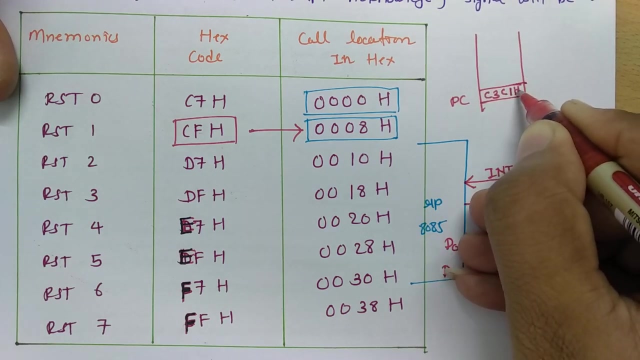 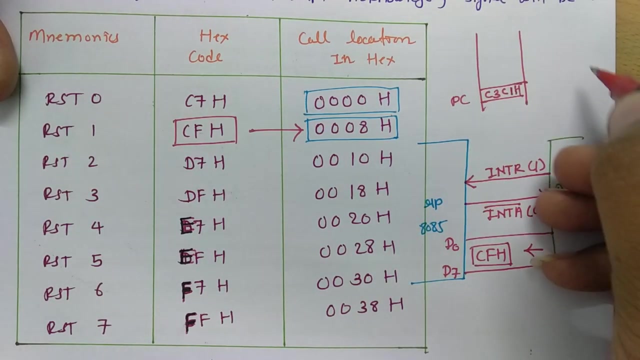 It means this processor that will jump to this memory location 0008, hex. Now see if I say right now, before this interrupt, if program counter that is there at C3, C1, hex memory location right, Then this program counter before it transfers control, this program counter that will get stored in stack. 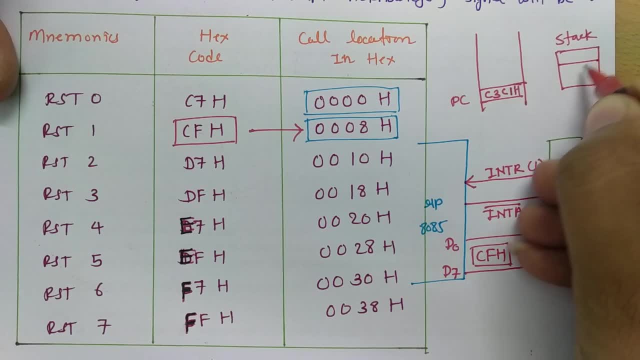 See if I say this is stack, so in stack at first C3 hex- data that will get load, and lower address C1 hex data that will get load, And then program control that will get jump at 00 hex. See here initial to data that one can see. 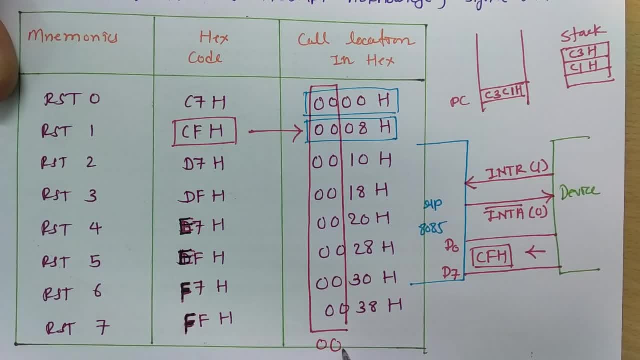 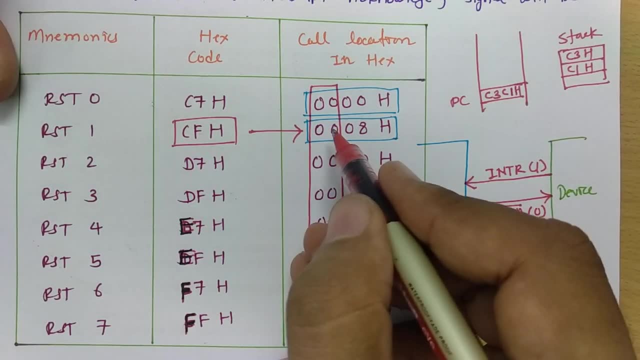 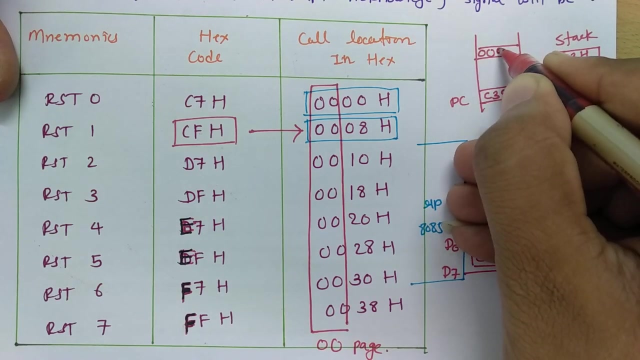 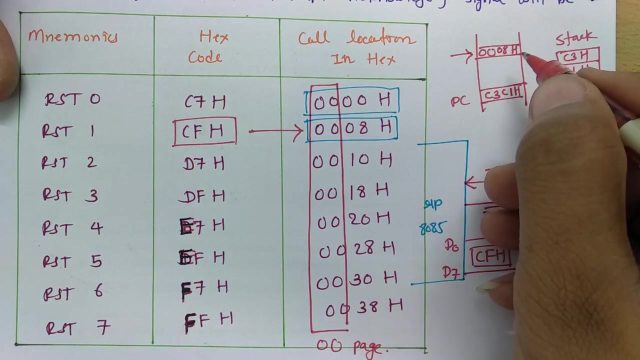 That is 00 means it is what 00 page And for this CF location is 0008.. So program control: now that will jump to 0008, hex. So now program control will be over here And it will provide service to this interrupt. 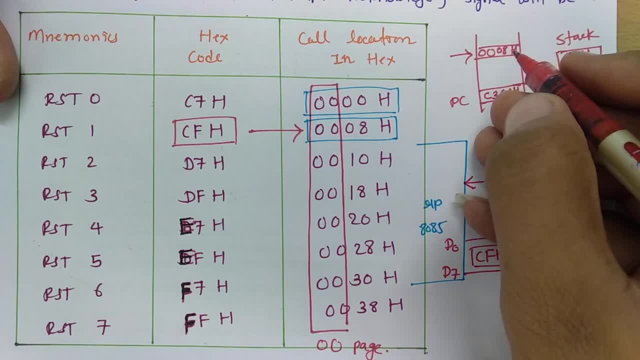 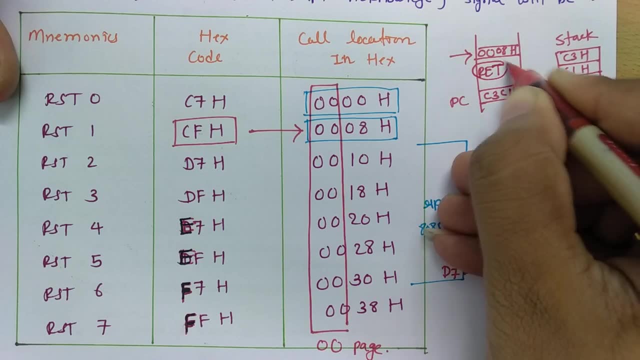 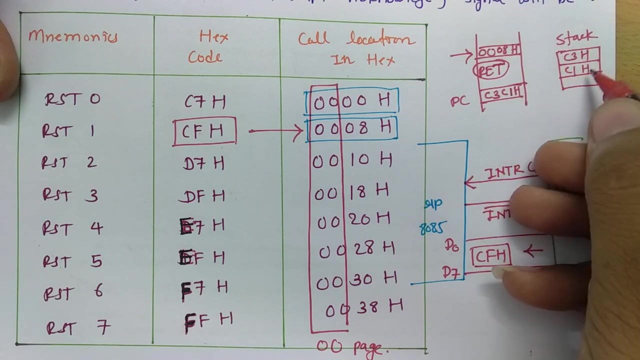 Once service of this interrupt is completed, At the end there will be return instruction, RET instruction, So as this RET instruction that is getting executed, program counter will load its original data from the stack And again it will come back to here.